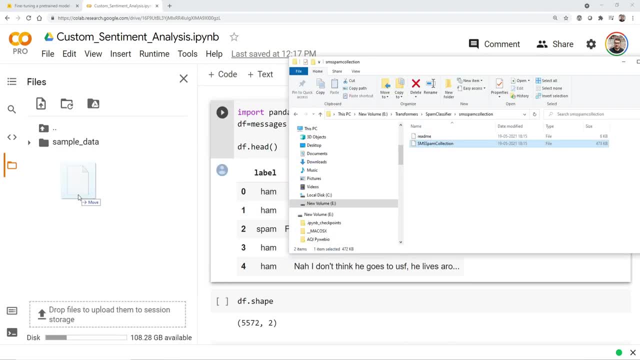 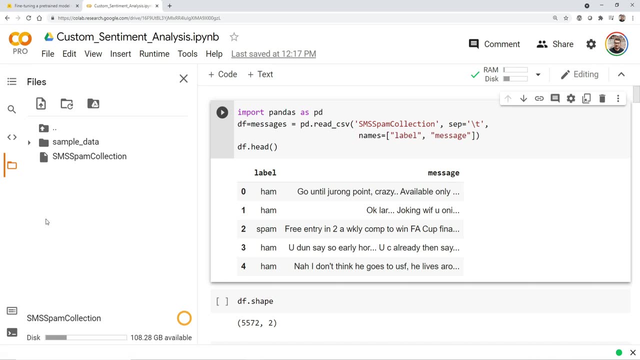 first of all, I'm just going to upload the data set over here, So let me upload it quickly and remember when you're uploading it. I'm doing it in Google Collab Pro, guys, You can also do it in Google Collab, So let's proceed. This is the data set over here, So this is. 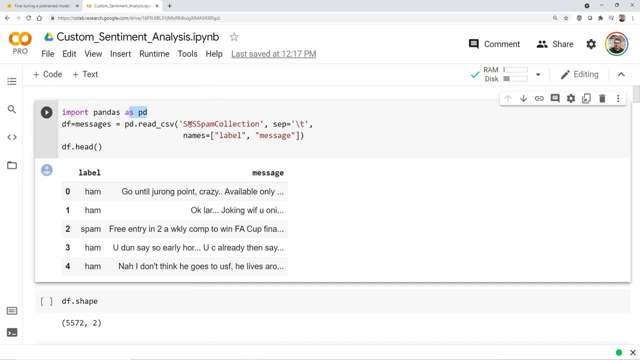 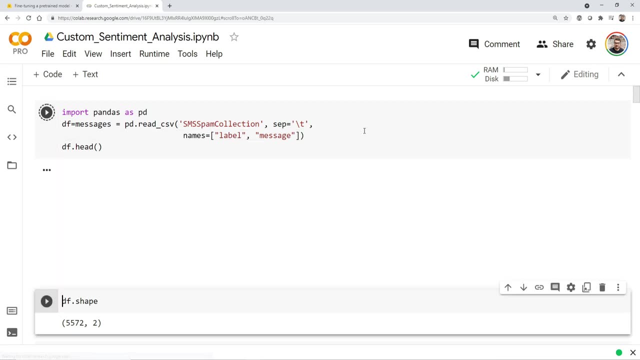 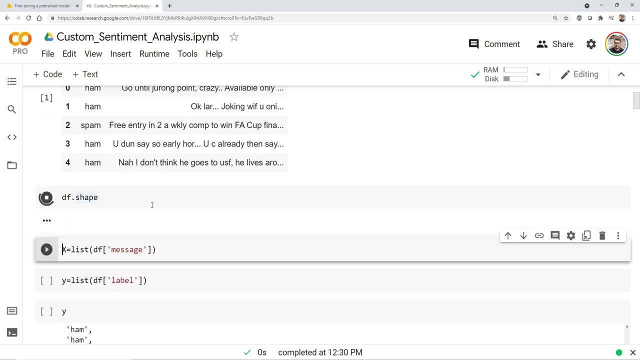 the data set. Now I'm going to import Pandas SPD and I'm reading this particular data set with a separated tab as this, and these are my two features, right? So once I execute it, you'll be able to see dfhead. and this is all my data set. If I want to go and see my dfshape, this is my entire data set of. 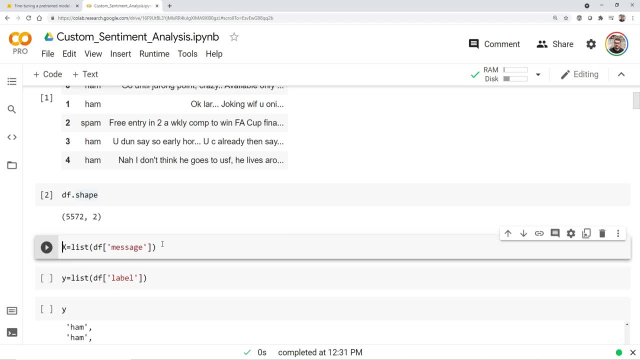 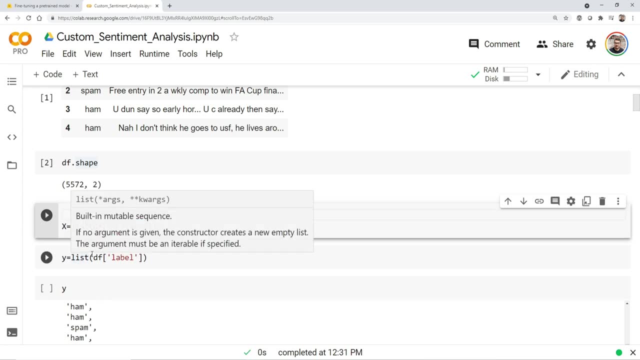 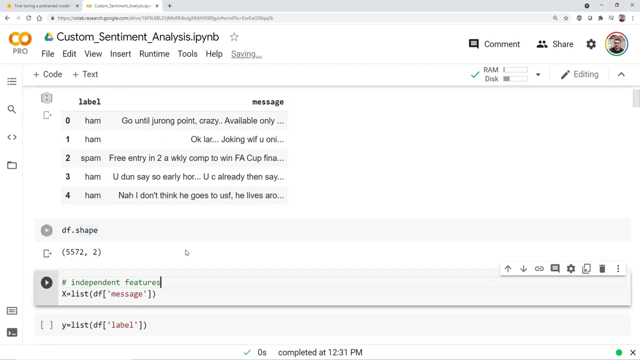 5572 rows and two columns. Okay, And then in the next step, I am actually converting this into independent and dependent features. So here is my independent features. Okay, independent features. And this, the other one is my dependent features. and red pill. tell you guys, once I take this df of message, I'm converting this into list. 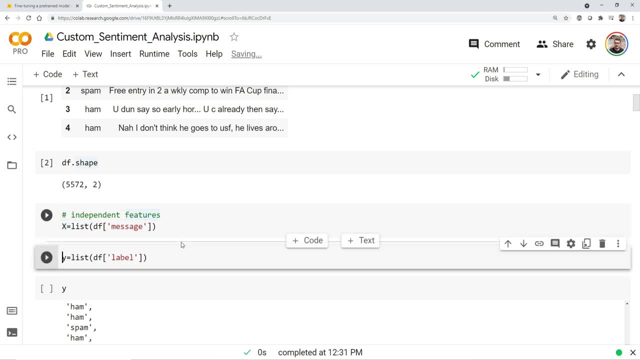 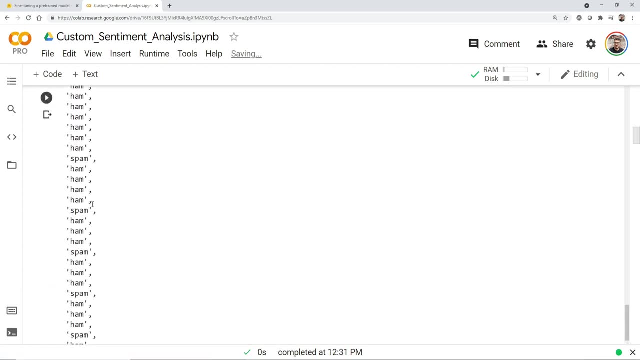 and storing it in my x variable. So let me just execute it And this is my y variable. Okay, converting into a list. So if I go and see my wife, so it is nothing, but it is having two categories like ham and spam. Now, before I go ahead with this, what I really need to do, this ham and spam. 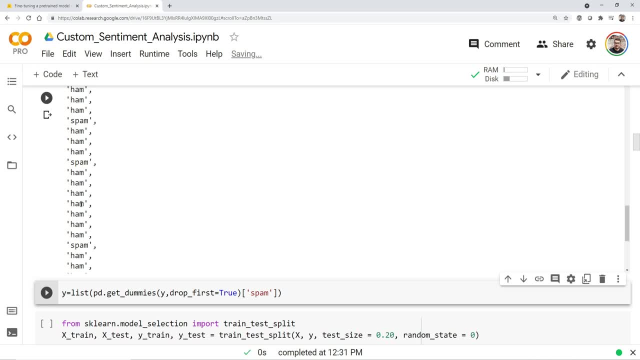 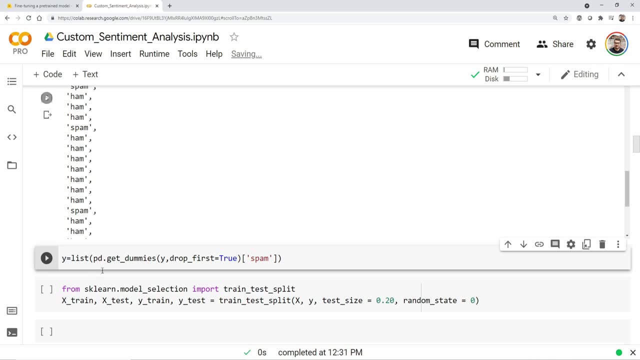 I'll try to convert this into zeros and ones, because I cannot keep my dependent features in ham or spam, Otherwise the model will not be able to understand. So in order to do that, what I'm going to do, I'm doing to do pd dot, get underscore dummies. y comma drop is equal to true with spam. 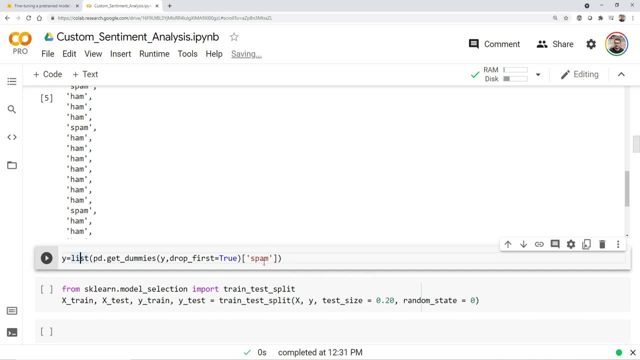 And I'm going to take the spam column and basically convert into a list. Okay, Because if I just execute something like this, see this, I'll just show you. So let me do one thing, Let me just create a code. If I just execute like this, you'll be able to see, I'll be getting one column with spam. Okay, so 001, the one that 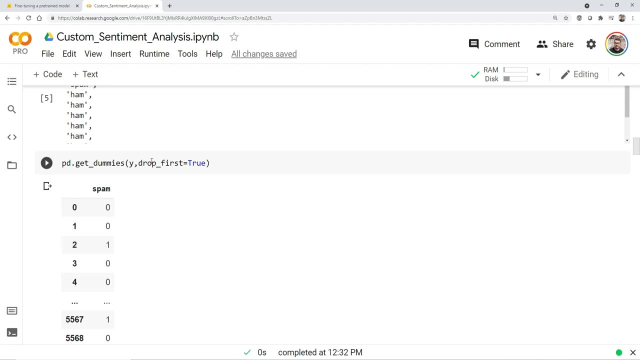 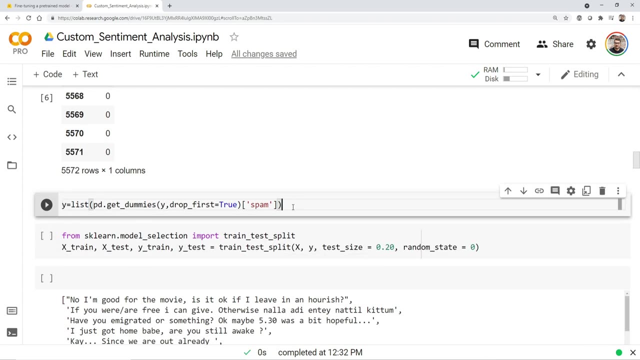 basically means when it is zero it is ham, Otherwise one it is spam. Okay, because I'm actually using like this. So I'm going to pick up this particular column and convert this entire things into list. That is the first. 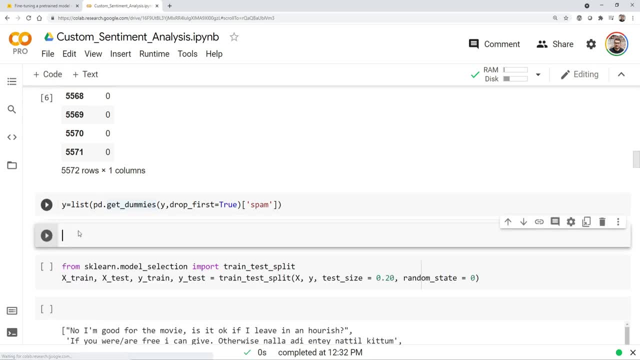 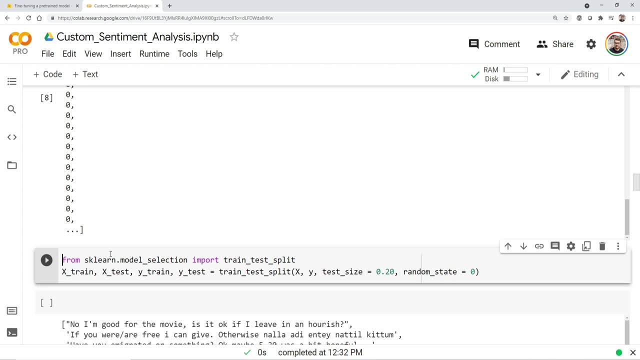 thing over here. So that is what I'm doing Now. if I go and see my y here, you'll be able to see that it will be a list, Okay, list of zeros and ones. Perfect. Now let's go to the next step. Obviously, this step is very much simple, not that difficult. doing a train test split. 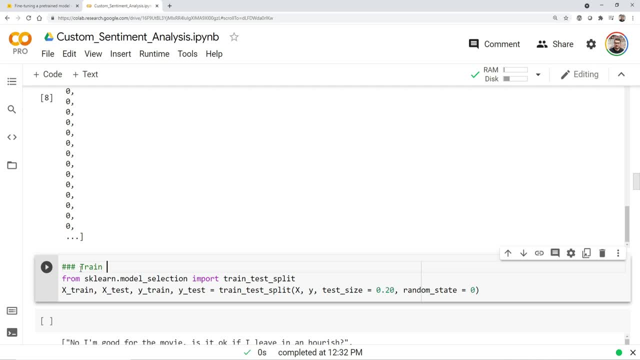 Okay, so here I'm just going to write it out: train test split. So if this entire thing I'll be giving you guys, because many people were asking how we can fine tune a custom model, So that is why I'm executing it. So, train test split, I've done it. 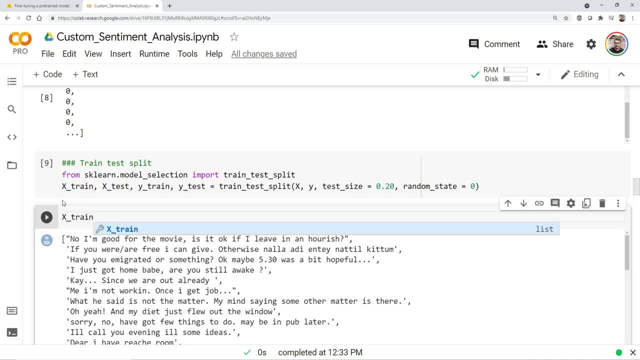 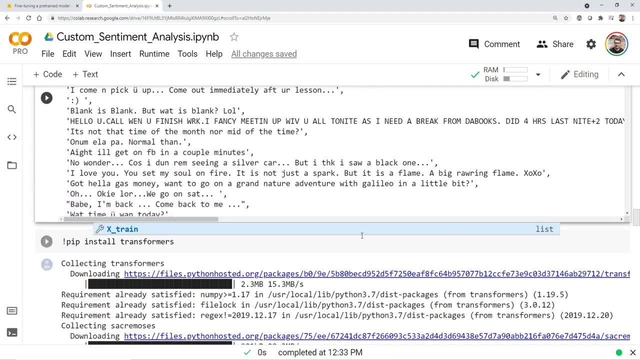 If I want to go and check out my extreme, I can definitely check it out Here. if I execute, this is my extreme entirely. So these are my features. Okay, Now, coming to the next step. we are going to install the transformers, because we will be using a model of 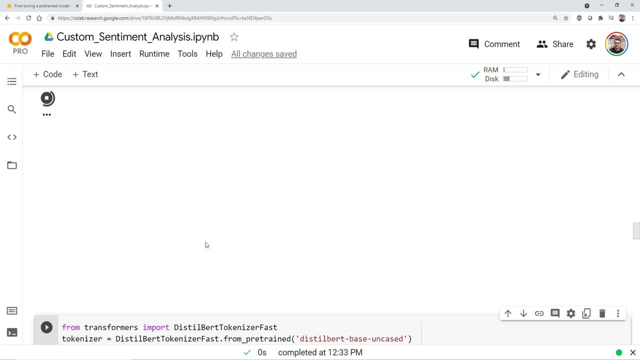 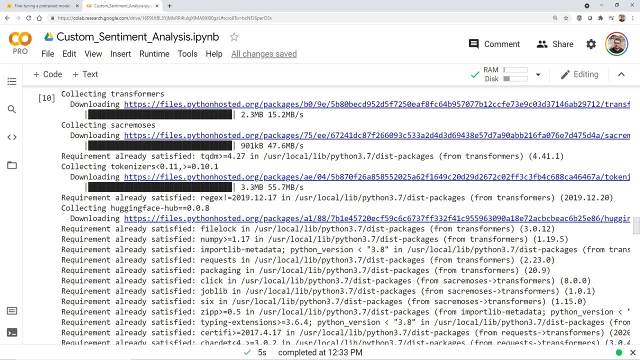 transformer itself, right, like distal bird. So let's pip install transformers. So here you'll be able to see the model will get downloaded. After the model gets downloaded, here you can actually sorry, after the library gets downloaded. Now you can basically. 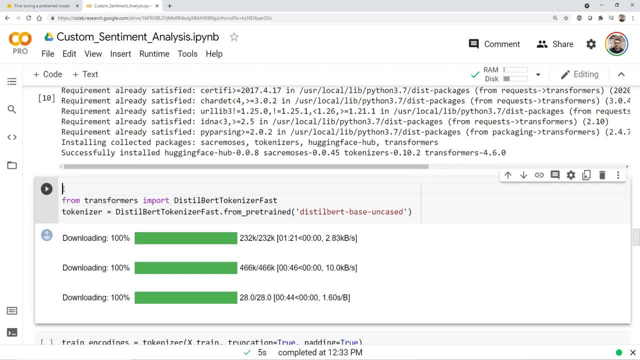 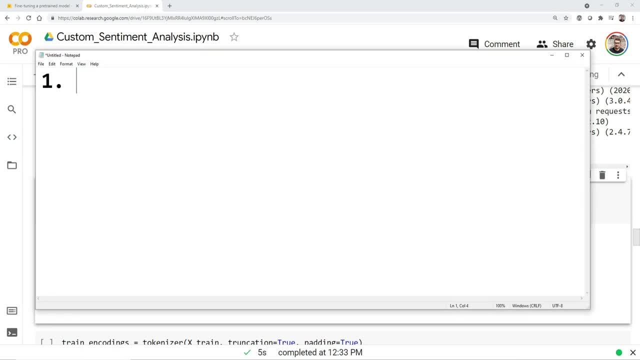 call the transformer. Now see, guys, what are the steps. Okay, with respect to transformers, I'll open a notepad. Okay, so that you'll be able to understand the first step after installing transformer. call the pre trained, call it a pre trained model. Okay, So call the pre trained model. the second step will basically be called the tokenizer. 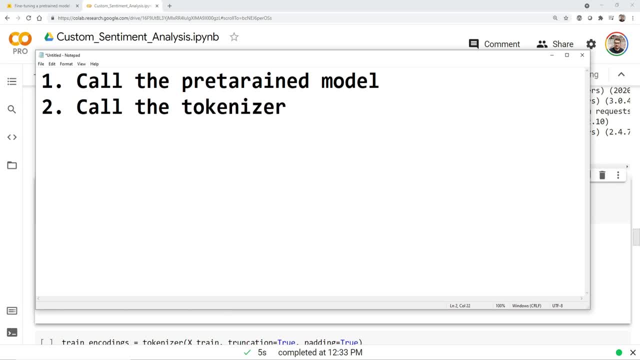 Because this tokenizer I need to apply for my data set also. And remember, guys, for a specific pre pre trained model, there'll be a specific tokenizer. Okay, suppose if I'm going to use my distal bird, okay, I have to use the tokenizer. that is with respect to distal bird, Okay. 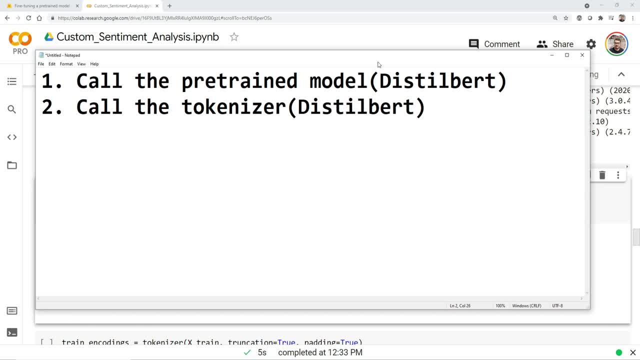 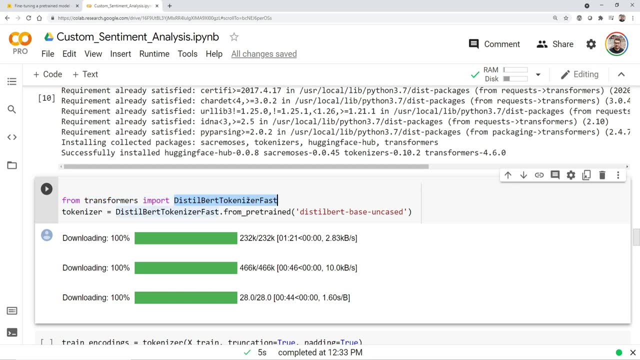 All these things, you really need to consider it, Okay. so in order to do that, I'll go to my file over here. So here you can see, from transformers I'm going to import distal bird tokenizer fast. So this is the tokenizer that will be used for yeah. and then I'm saying: 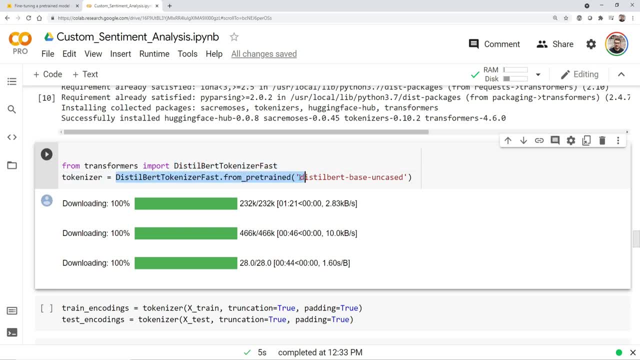 tokenizer is equal to distal bird tokenizer fast from pre trained on distal bird on cased okay. So similarly you'll be having different, different tokenizers. okay, all together distilbert. i would suggest take up this particular tokenizer again. you can explore the tokenizers. 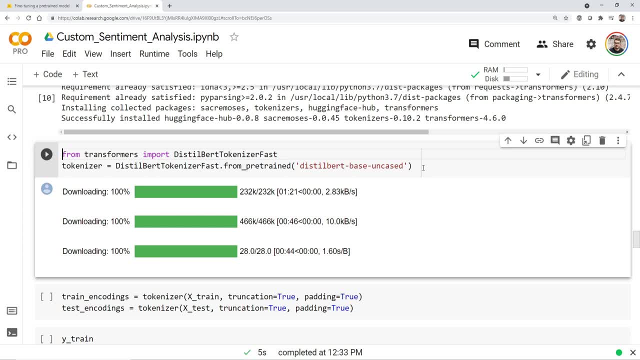 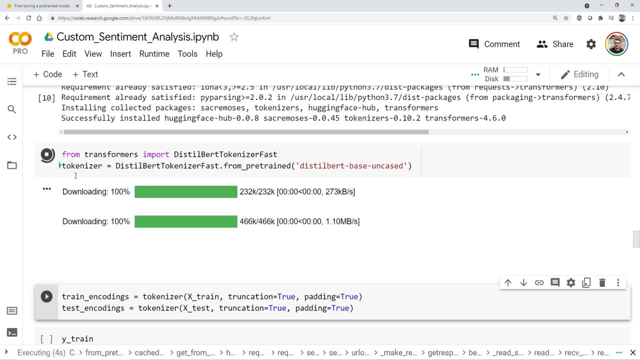 in the documentation page of the transformers, then i'm going to use this and try to execute it. okay, so this is my tokenizer, which will be responsible for tokenizing or converting my sentences into some numerical values. okay then, here you can see i'm giving my tokenizer, i'm 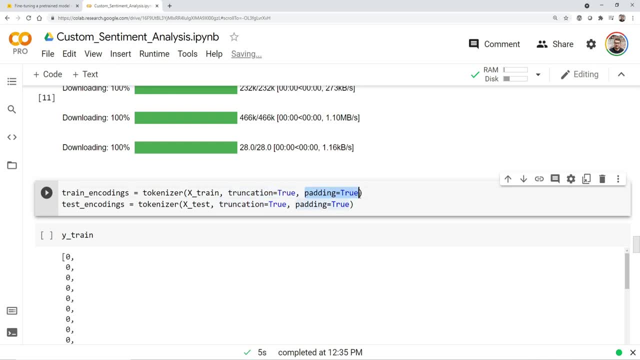 giving x underscore train. truncation is equal to true and padding is equal to true. this two are actually done. if i go and see over here, truncation and padding are actually usually done. see, padding is usually done to make all the sentences of the similar size. truncation is to: 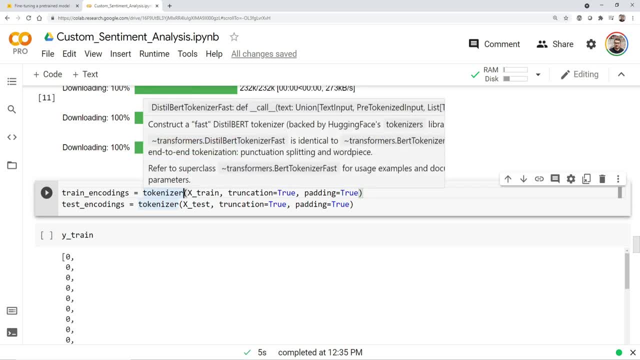 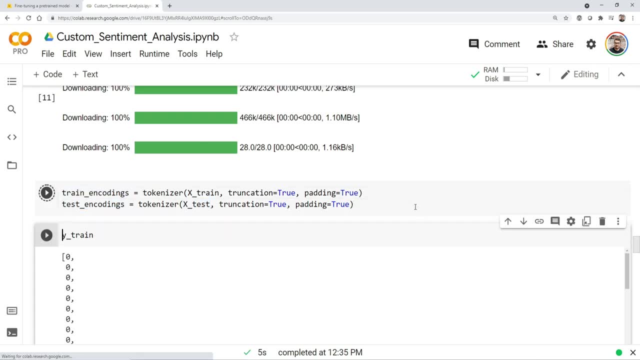 remove the white space. okay, so all these things is done. so here you can see it is done for both x train and x test. so there i'm getting train accounting and test encoding. so once i execute it- okay now if i go and see my train encodings here, you will be finding some amazing things okay. 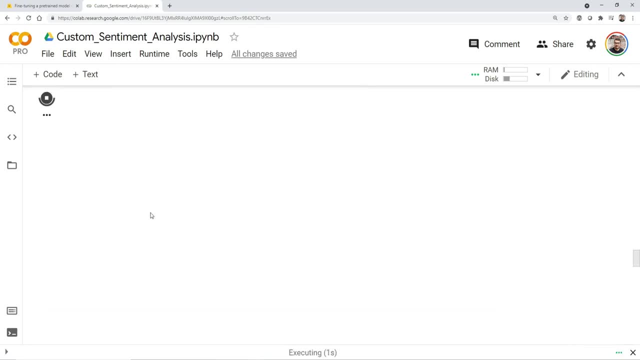 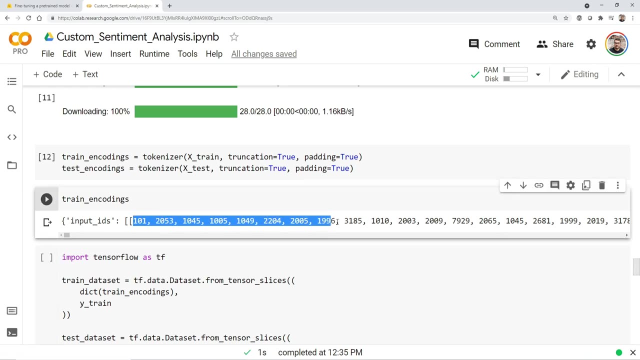 as far as i remember, here you'll be having input ids, here you'll be having the master id, everything. so if i execute this, so here you can see i'm getting my input ids. this is my numerical values with respect to the sentences that i've actually given, and see here, this is all padding, okay and by. 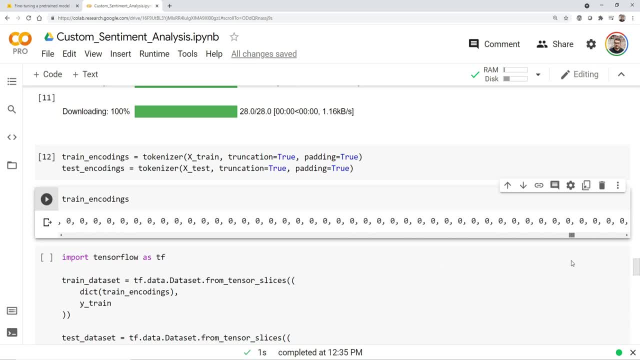 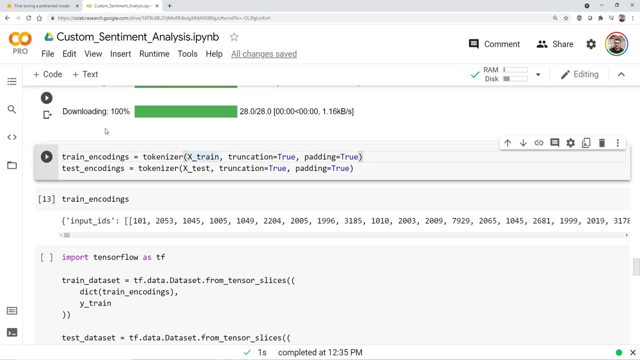 default, i think the size is 512. okay, you can also give your own size. it's not like you just have to give the same size. you can give your size with respect to anything that you want. okay, probably, you want to give at 100. okay, instead of 512, you can give it. okay, by default, this takes 512.. if you want to see this, 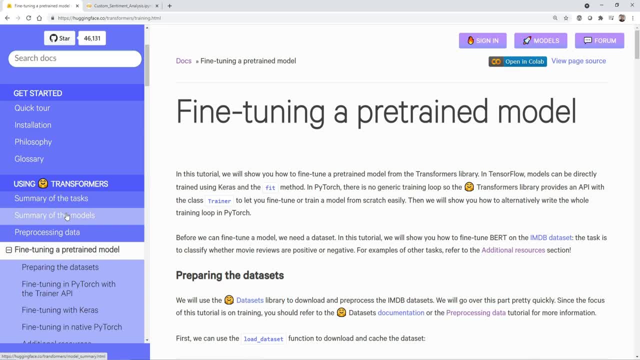 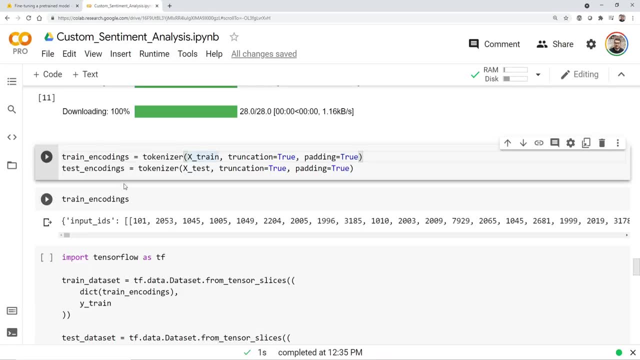 just go and check in one of the quick tour or summary of the task. there you'll be able to find how to, how you can basically give up the values, or you can also check out this particular page. okay, perfect. so this is good. we have found out the training codings and testing codings. i have my 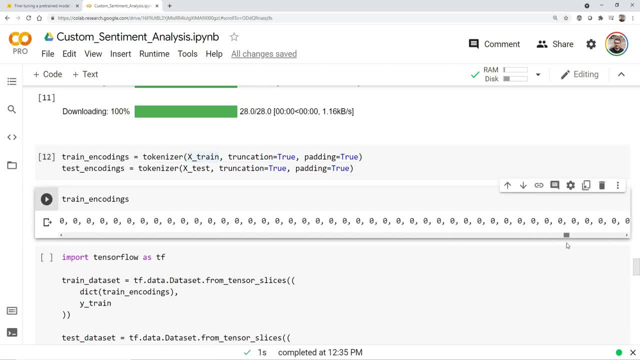 input ids completely with us. so this is perfect. now let's go and check out what is the next step. okay, now, in the next step, we're going to give you a task. okay, this is very difficult to give a task. okay, now let's go and check out. uh, what is the next step? okay, now the next step. we have to give a task. 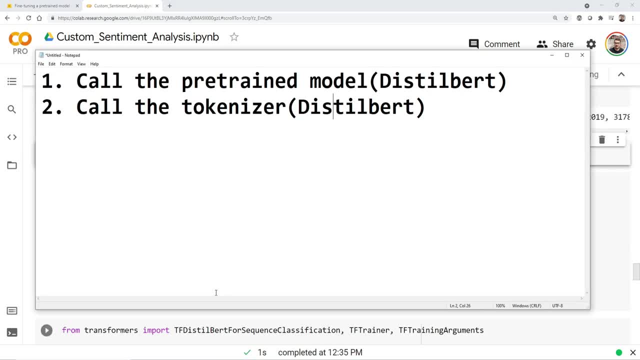 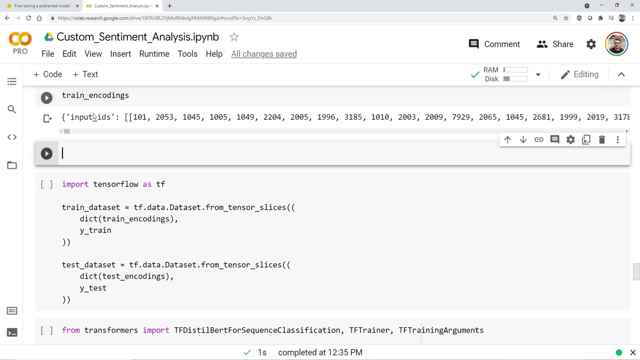 next step is also very, very much important. let me note down in a notebook file: okay. the next step is that we really need to convert these encodings, these encodings, into data objects, data set objects. what is the data set objects? i'll talk about it in case of, in case of, uh, when? 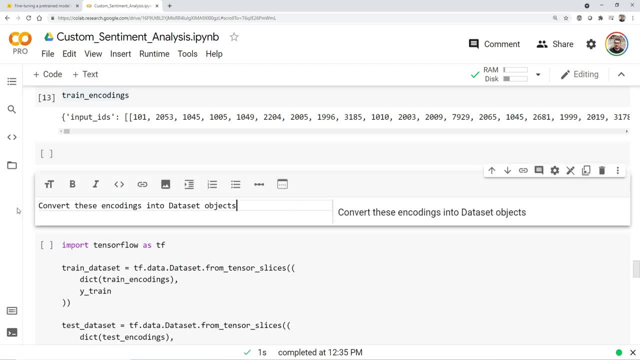 just let me write it down. okay, in the case of what happens is that when i'm using transformers- see over here- when i'm using this transformer, i'm going to use tensorflow. okay, if you are using pytorch, then it will be a different data such object. in the case of tensorflow, it will be. 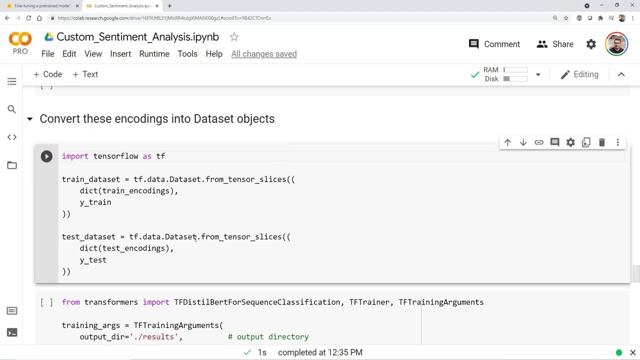 tensors, you know. so we really need to create in the form of tensors. so for doing that, here is what i'm doing: tfdataset from tensor slices. i'm giving the dictionaries. you know the training encoding in the form of dictionaries and my y train value. similarly, over here i'm giving from a testing. 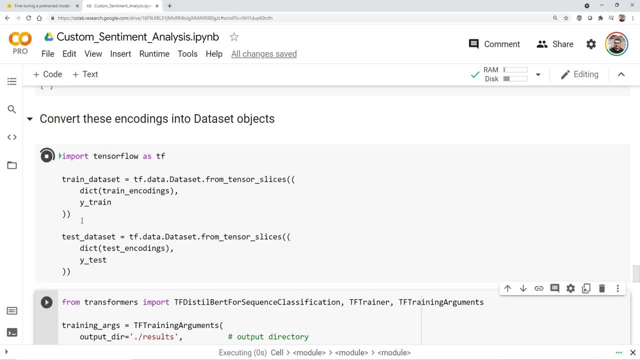 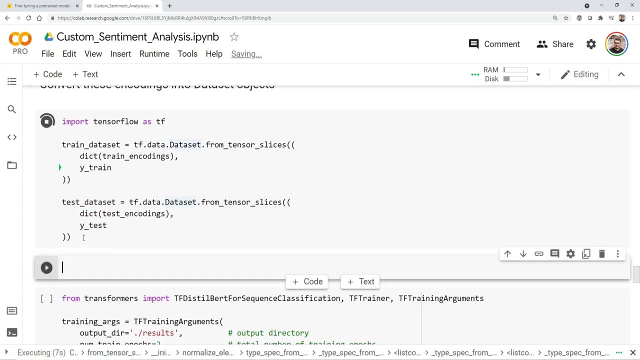 value and i'm giving the training encoding in the form of the training encoding, in the form of encodings and y test values. so if i execute it here now, you'll be able to see what will be the format. okay, so this will take some time because i have a huge data set, so i'll just make this one. 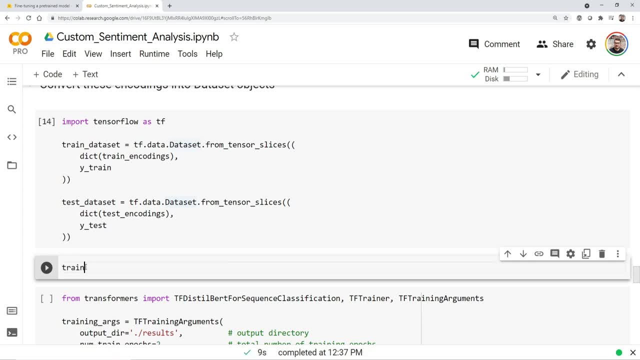 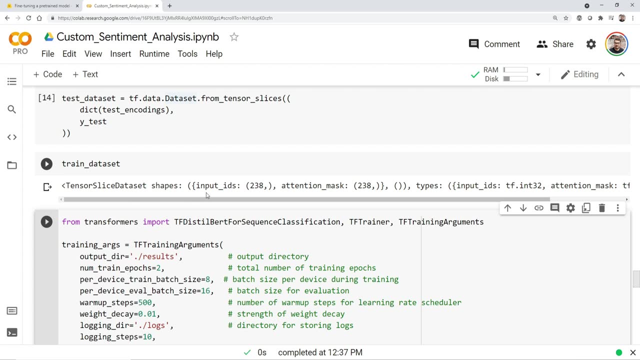 and probably just try to show you how my train underscore data set looks like. okay, so once i execute it, guys, here you'll be able to see. it will be in the tensor slice shapes. the input ids will be there, attention mask will be there. this input id is the attention mark. all all this particular. 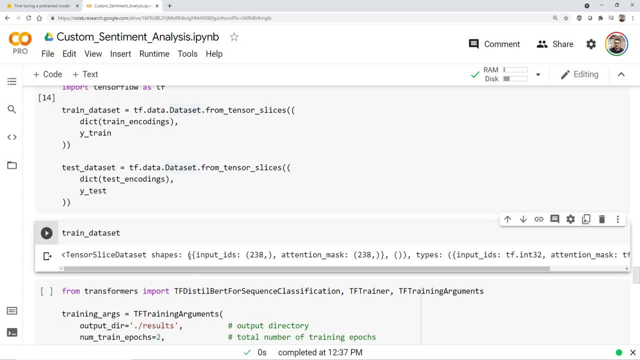 information, because this is the way to do it. so i'm just going to show you how to do it. so i'm going to show you how to do it. so i'm going to show you how to do it. so i'm going to show you format that the classification sequence, classification that we'll be using. that is, 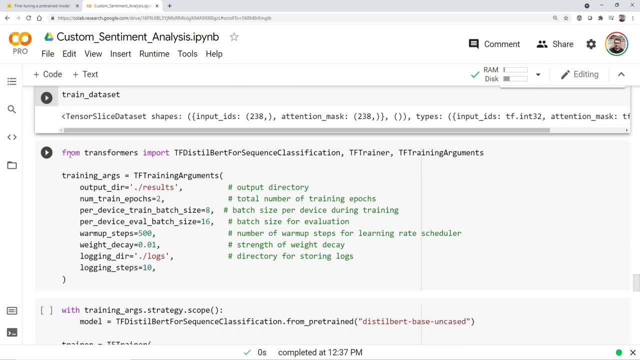 the distal bird now coming over here. guys, the next step over here. you can see that from transformers. i'm going to import this sequence classification. remember the sequence classification is mostly for sentiment analysis, not for question answer, application or any type of sentiment analysis that you really want to do. you really need to import the sequence classification library, okay. 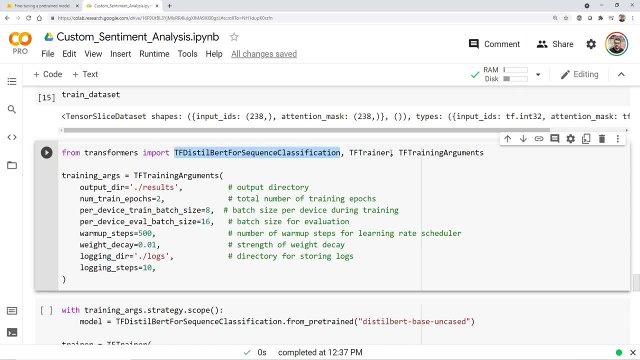 so i'm using df- distal bird for sequence classification. tf- trainer and 3f- training arguments will be responsible for training my model. after my model is basically trained, i'll be using this tf trainer object to do the prediction. so i'm going to use this arguments over here. my output directory will: 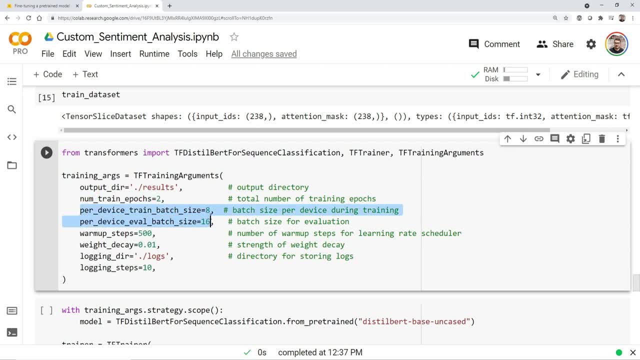 be results. number of training epochs will be two per device. train batch size will be eight, remember, try to make it as 8 and 16, then only you'll be able to run it in your google collab. probably, if memory out of error is coming, you try to reduce into four and eight warm-up steps. 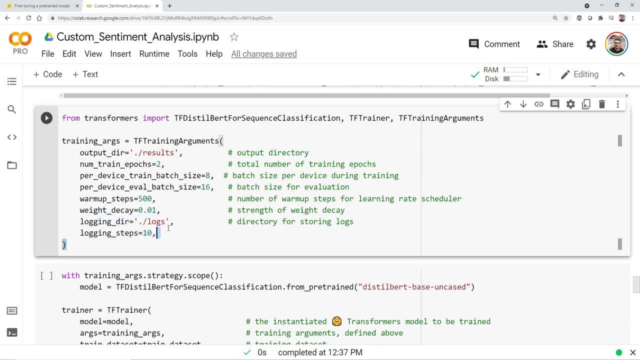 will be 500 and then all my logs will be stored over here. logging steps will be 10. okay, these are some of the information that i'm giving over here. okay, all this particular information are just some kind of parameters, so let me just execute it now over here. you will be able to see that i'm going. 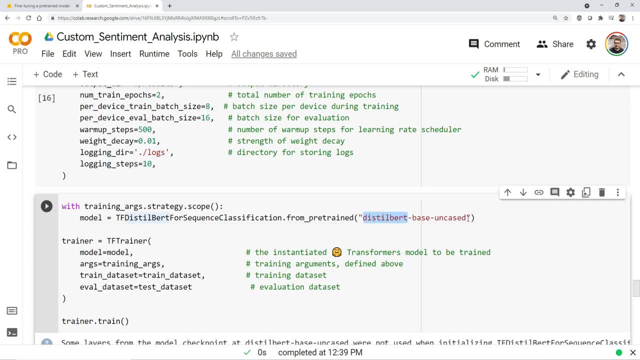 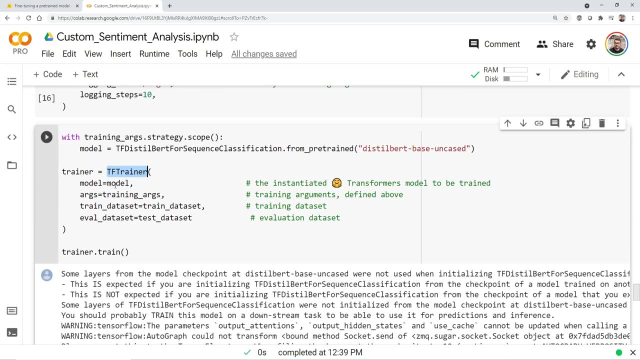 to use this distal bird for sequence classification from pre-trained model distal bird, uncased. okay, and then i'm actually starting my training by the help of 3f trainer, where i'm giving my model value over here, argument, training arguments, whatever training arguments i've created over here. 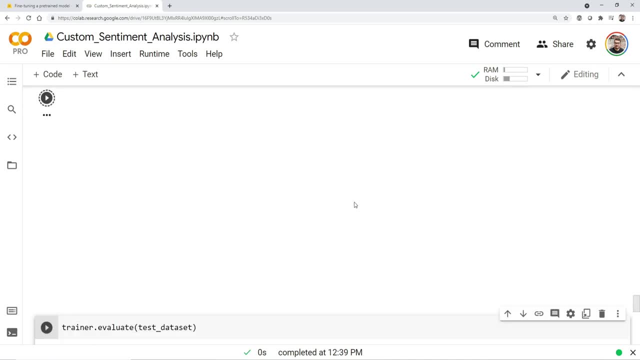 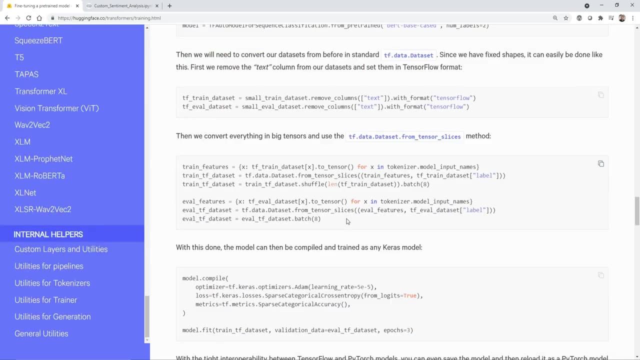 my train data set, my trash data set, and then i do trainer dot 10.. now you may be thinking: krish, how do you know all this thing? i, i i'm just following this documentation, guys. that's it okay to do my custom things. you can also do it in pytorch, you can also do it in tensorflow. remember these things. 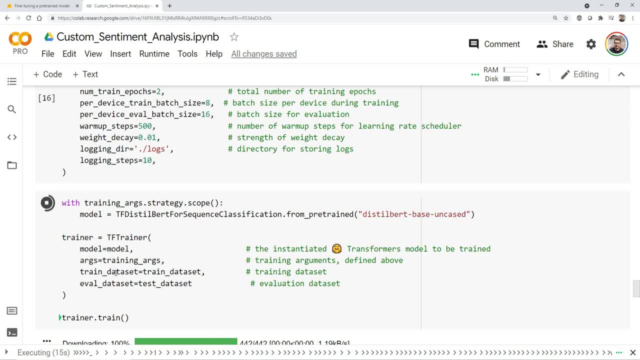 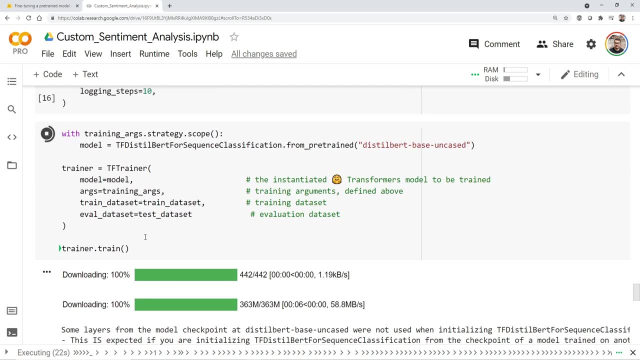 will not change, because this can, this can be used for any kind of data sets that you are actually planning for. okay, any, any kind of data set, whatever data set you have in your mind, you can use that with that specific data set and you can do it. okay, now this will probably be a little bit. 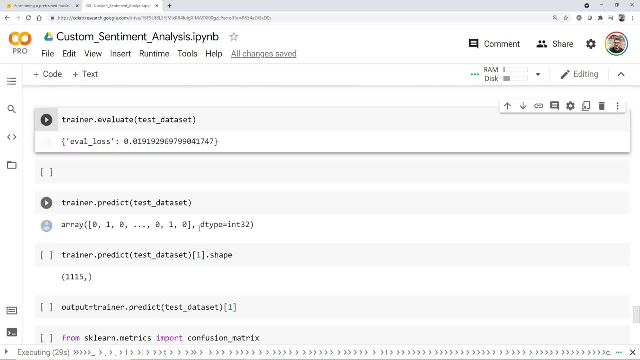 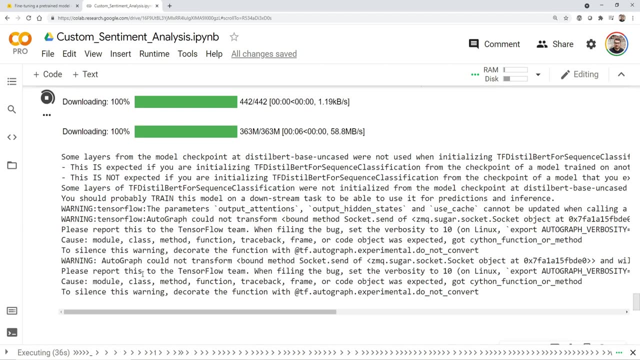 more complicated, but it will probably take some time. uh, till then we'll just wait and then you'll be able to see. we'll be able to evaluate it, predict it with respect to a test data and all, but remember whenever you really want to predict it with the respect to the new data, again you 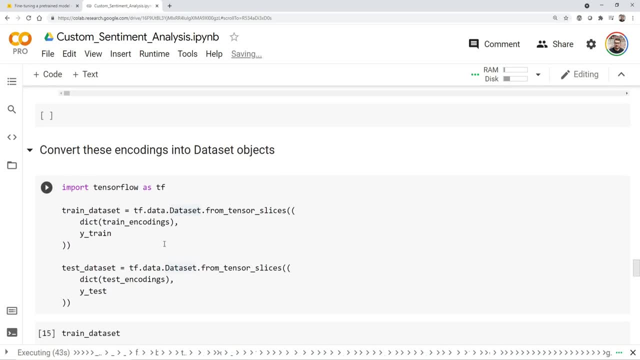 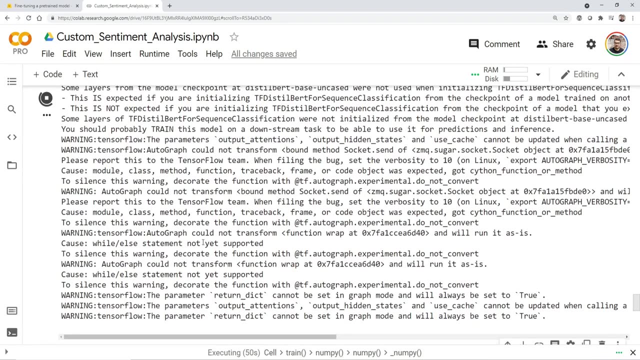 have to do all these things, that is, your tokenizer and your encodings. okay, you really need to do this, and then only you'll be able to find out the output. perfect, so we'll wait, uh till. uh, this entire thing is getting trained. it will probably take some time, and here i've just taken 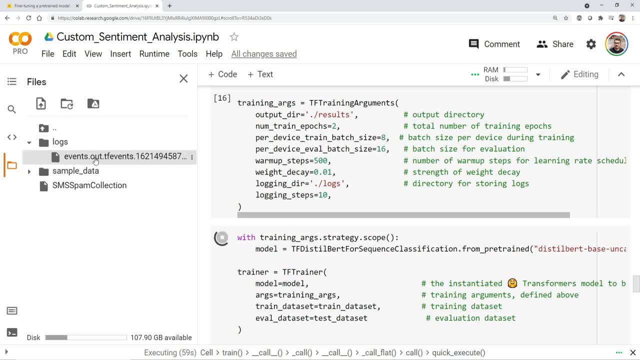 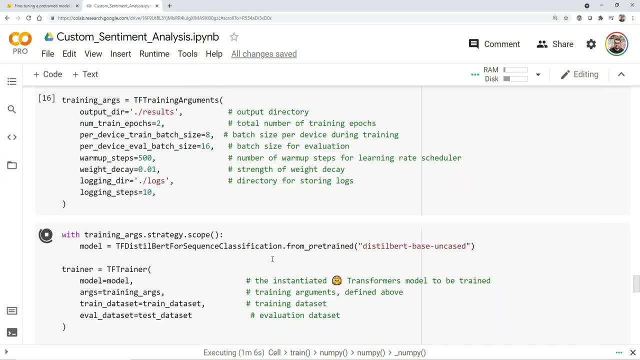 let's see whether the folder has been created or not. so here you can see the logs folder has been created. so here is my logs folder. event out: tf events over here. so yes, let it go. these all warnings will be coming, you don't have to worry about it. 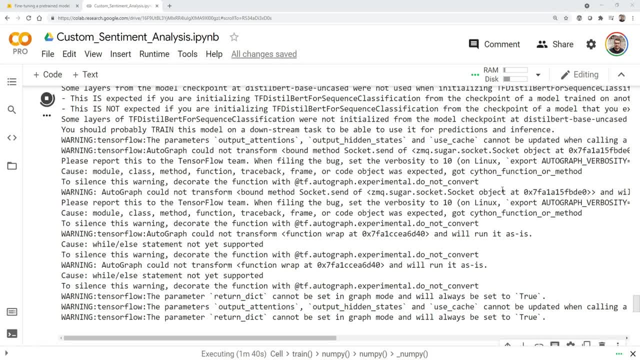 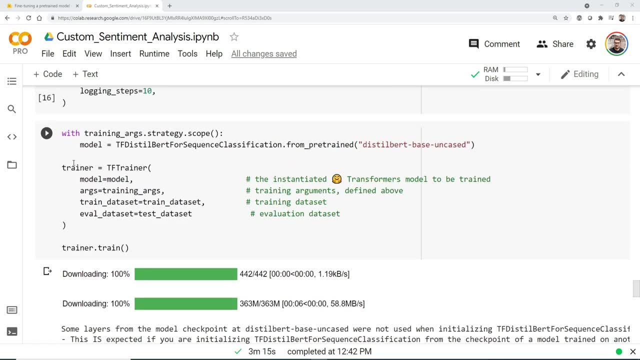 so let's wait, and let's wait till the training is done, okay, guys. so here you can see, the training has been done. okay, i've just run it for two epochs. you can also run it for four to five epochs, but approximately took me somewhere around uh, two. 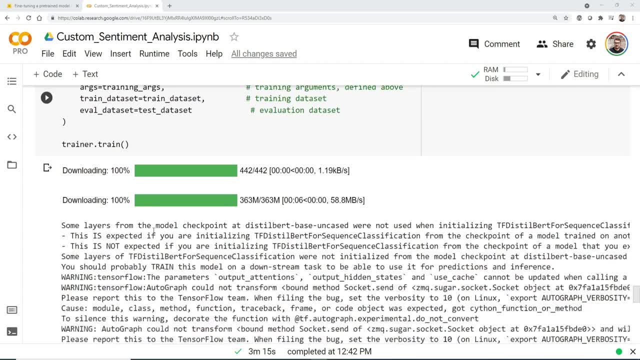 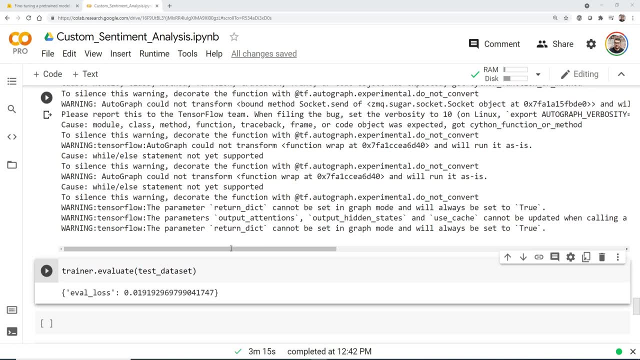 to three minutes. uh, probably in google collapse pro. now, if i go and execute trainingevaluate- so here you can see- my eval loss will be probably given some value. okay, so if you run it for two epochs, two minutes approximately. so now you can see. if i run it for three minutes, you can see. 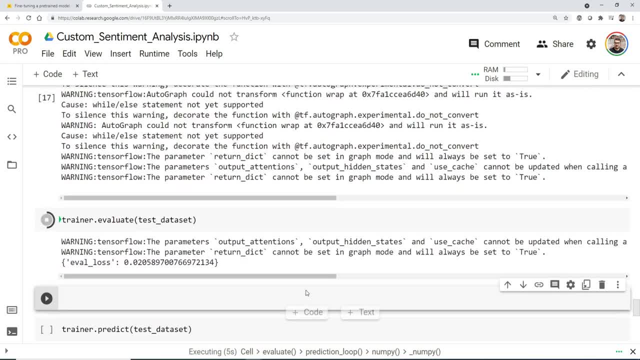 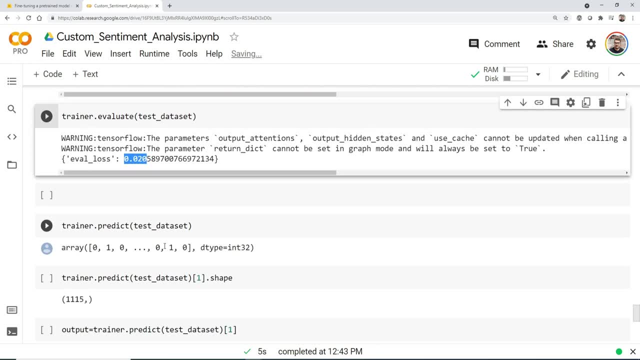 that it's not going to happen. something has happened, okay. so here, it took about a minute plus, so let me execute. so it is somewhere on 0.02, okay, so it is very, very less. it is almost near to zero. now, if i do the prediction in order to do the prediction, uh, i can, and why i'm using this. 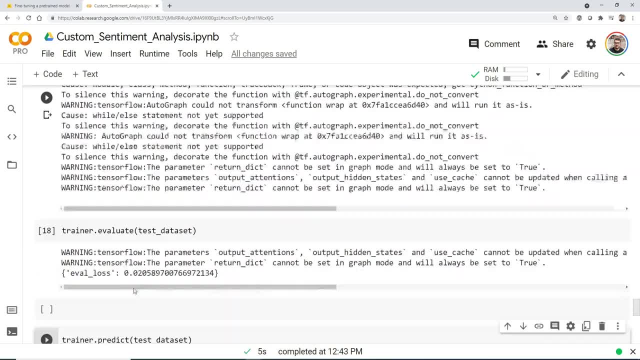 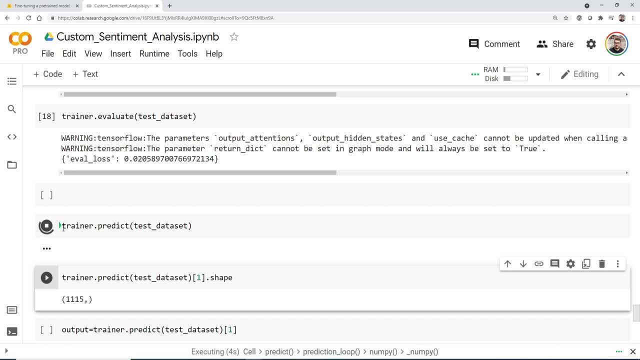 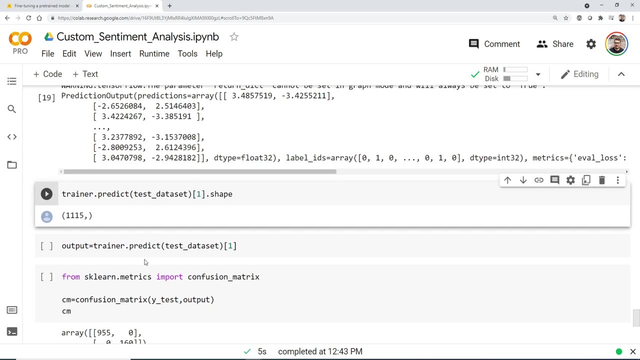 trainer- remember, this is my trainer right, which is actually trained. okay, so i can do now trainer dot: predict on test data set. okay, so here you can see all the predictions. okay, probably, uh, if you really want to check out the output. this is basically all my outputs that i. 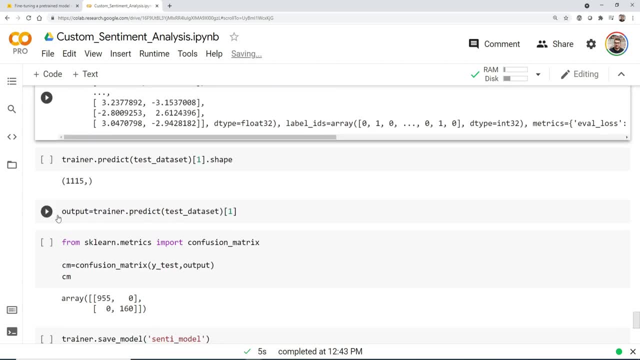 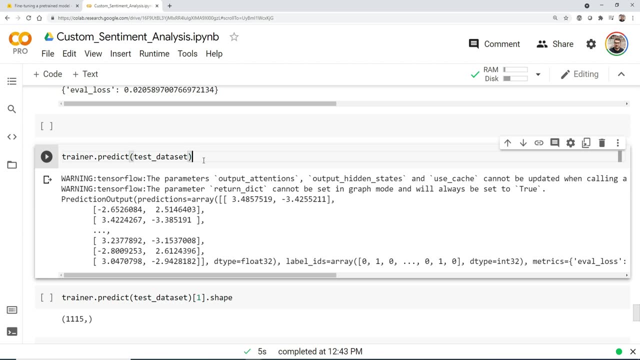 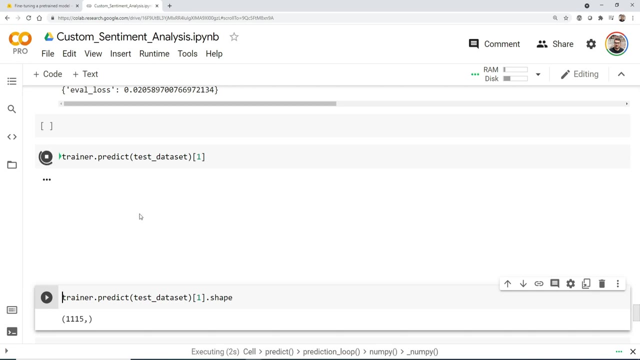 want. right, this is my all the outputs i want, okay, from this. so, in order to get these outputs, i can write trainer dot- predict test of data, which is this: if i just execute this one one here, you'll be able to get all the values you know, the prediction, probability, prediction- okay, and 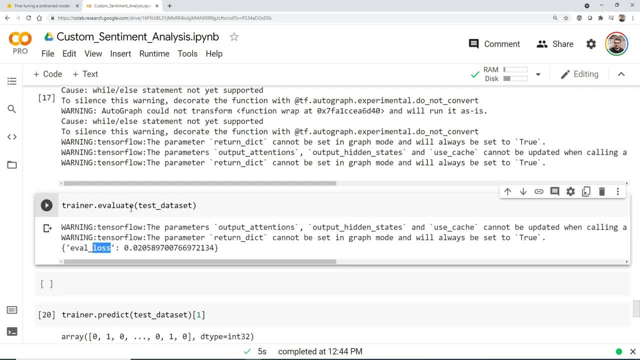 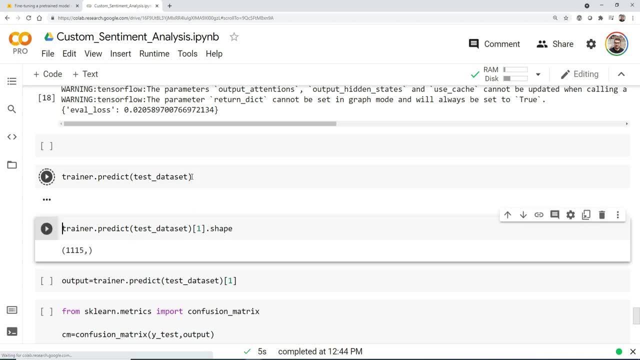 test data set has see all these things you are actually able to get. okay, did it go here? so this is what i want, i'm interested in. if i go and see this entire information here, you'll be able to see a lot of informations in shot. uh, you'll be able to see the. 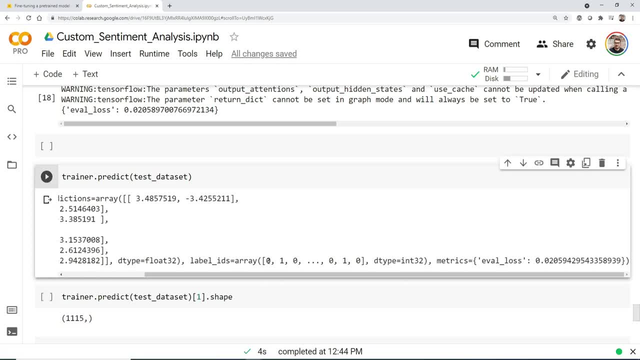 data sets. one thing is label ids, right, so label ids is nothing but your class, so i'm going to take up this. in order to take this, i'll be using an index of one. remember, this is all in the form of tuples, okay, so label id i'll be trying to take in order to take, i'll just use this one and this will. 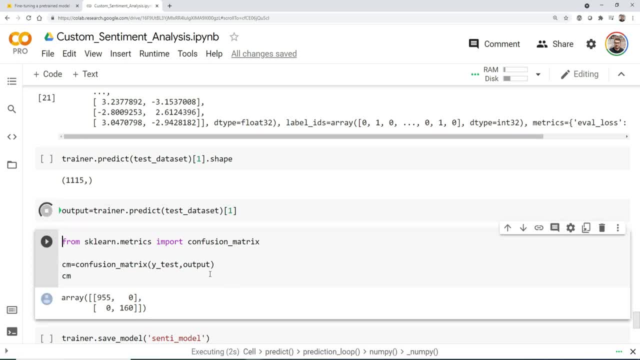 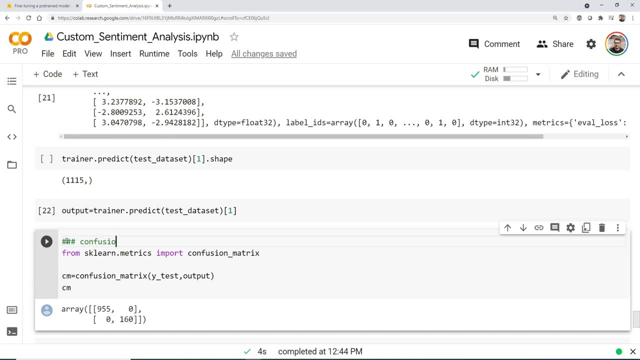 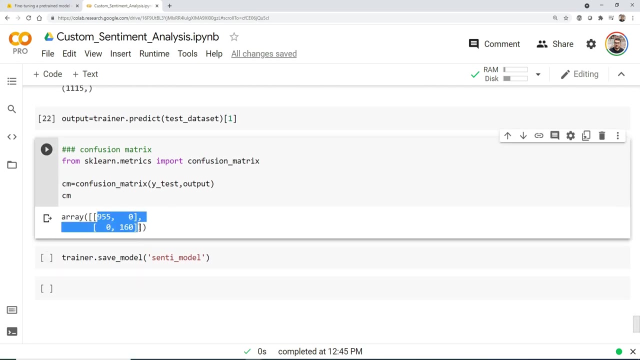 be my output, okay, and then after that, after this, i'm just going to create my confusion matrix. so this will be my confusion matrix, just to show you, like, how it has, how my model has actually performed. so definitely away, you are getting the accuracy of hundred percent. okay, it is pretty much good now what you 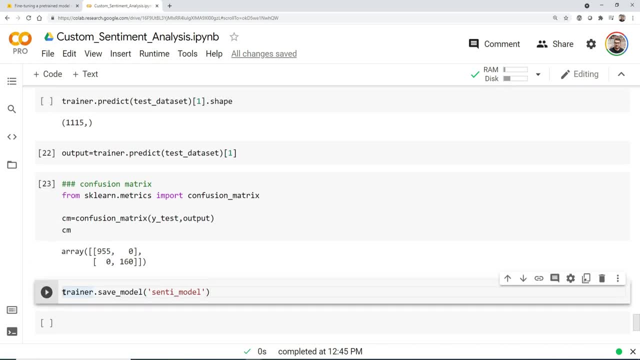 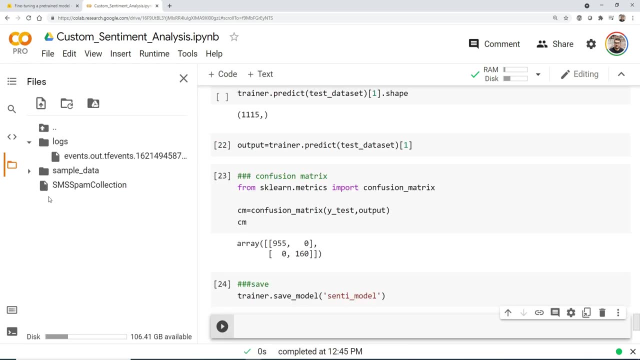 can do is that you can also save this particular model. so for saving this model, you just have to write like this and just write: trainer dot save senti model. it will basically get saved over here. so here is your results. okay, the checkpoints. everything is present over here with respect to 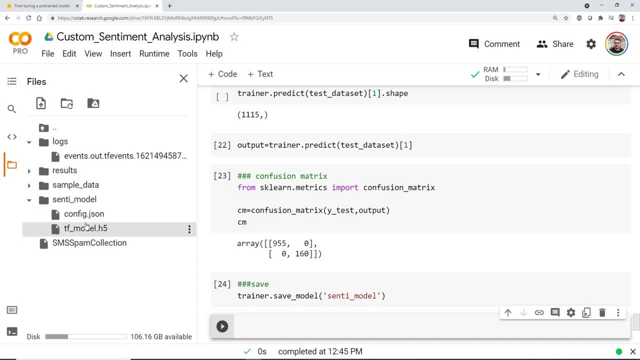 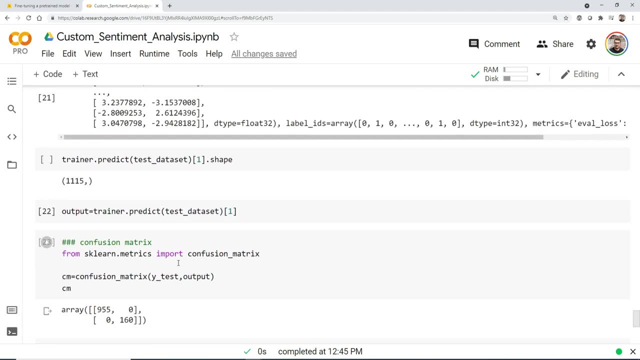 two epochs, two checkpoints, and then here is your senti model. this is your h5 file. now you can download this h5 file and use it however you want. okay, this is very much simple, guys. you have got the accuracy score, you have got the prediction. so let me also write a comment over here, right? 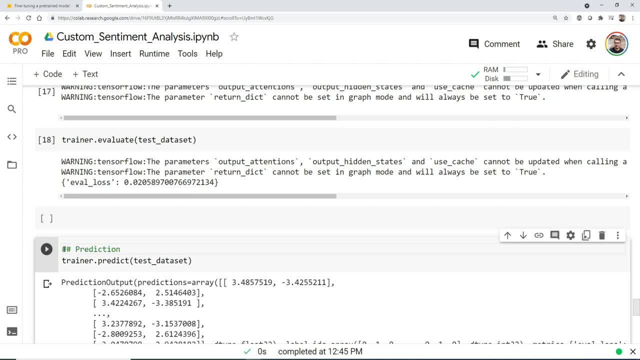 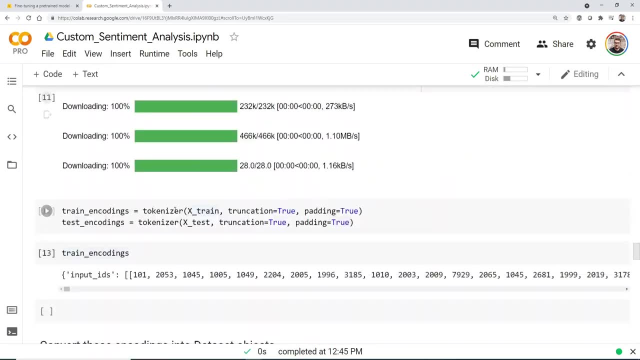 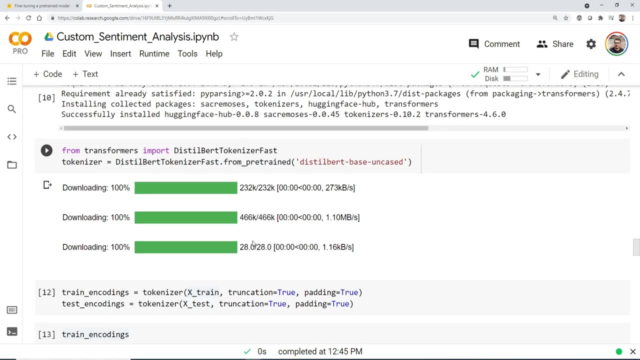 so this is very much simple. always remember you need to know what all things we actually did with respect to the encoding things you know. so we took the tokenizer of this one distilbert tokenizer fast. if you are using bert based uncased, then use bert tokenizer fast, okay, and then you have. 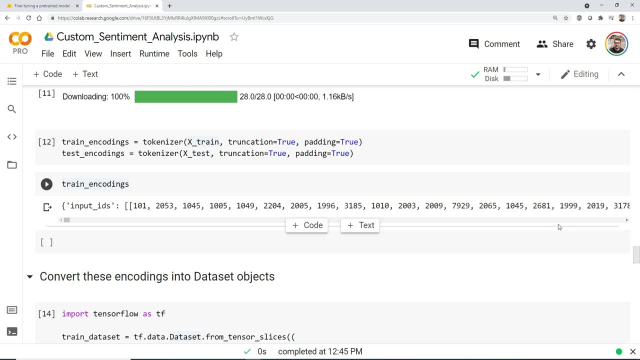 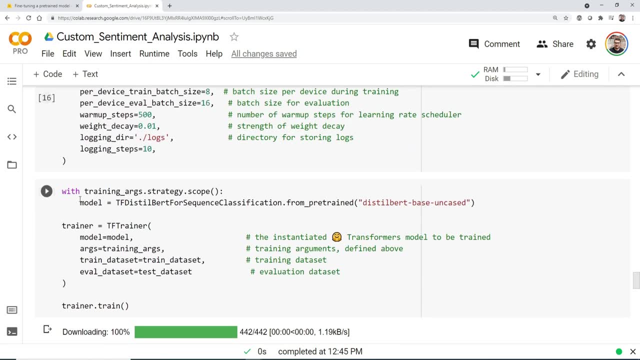 to use truncation, padding is equal to true by default, the truncation and the padding is nothing but 512 characters- and then convert this encoding into data set objects. in the case of tensorflow, it is tensorflow slices, and then all the steps are pretty much simple here. you are just saying: 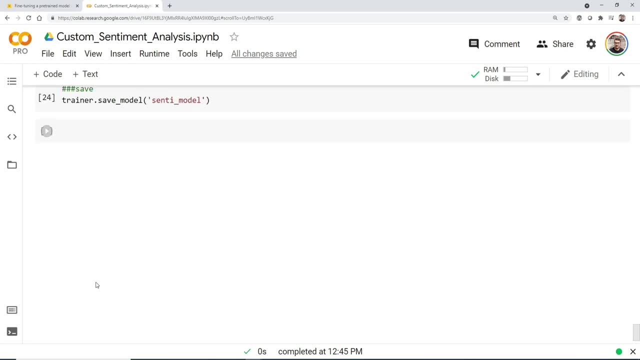 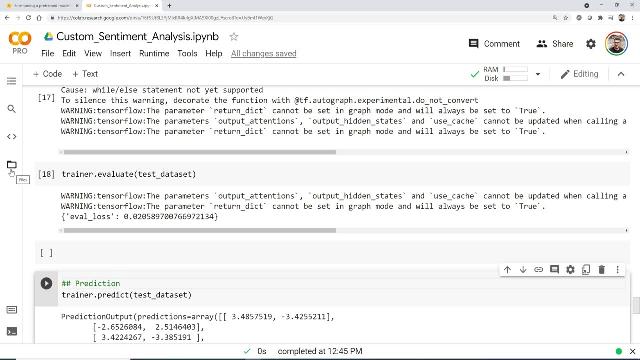 how many checkpoints you want and all these things. so i hope you like this particular video. now, what do you guys? i'm going to give you this entire file. along with that, i'm just going to give you the data set. so the data set, which is nothing but the spam collection. okay, so both this data set.